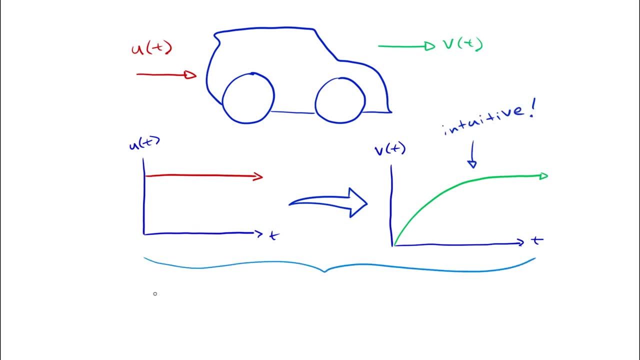 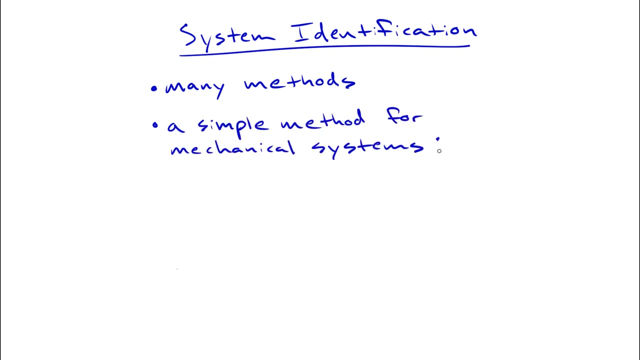 We knew this intuitively. We also learned that Simulink requires a mathematical model that captures the system dynamics. Fundamentally, the process of mathematically capturing a dynamic system is called system identification. There are many ways to identify a given system, but one simple way to model a mechanical system like this is to first analyze the external forces and then apply Newton's second law. 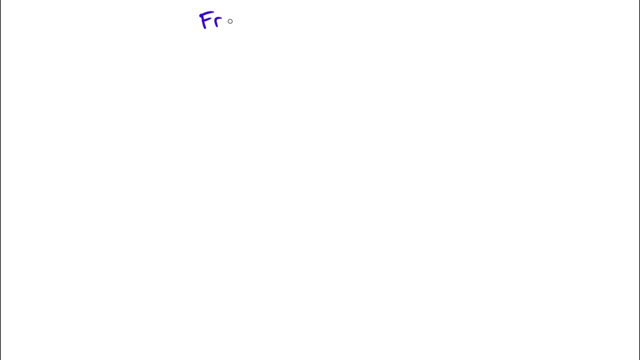 To analyze the external forces, a free body diagram is extremely useful. Since we're only concerned with the dynamics of the vehicle in the horizontal direction, we only need to consider forces in that direction. There's one force providing a forward thrust and another, aerodynamic drag force, which is often simplified as a proportional gain that scales the velocity. 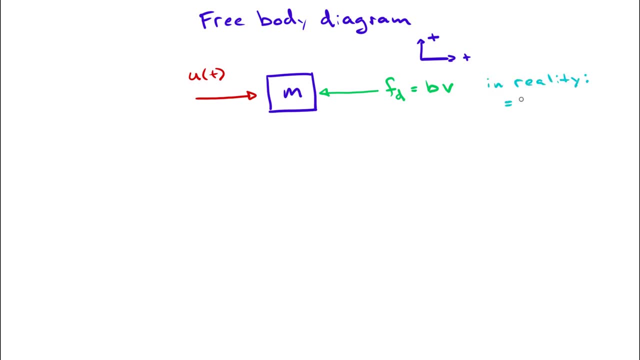 In reality this is a quadratic function, but a simple linear model serves to illustrate the modeling process here. Then we can apply Newton's second law to produce the following equation: However, we need to think about this equation in a different way. 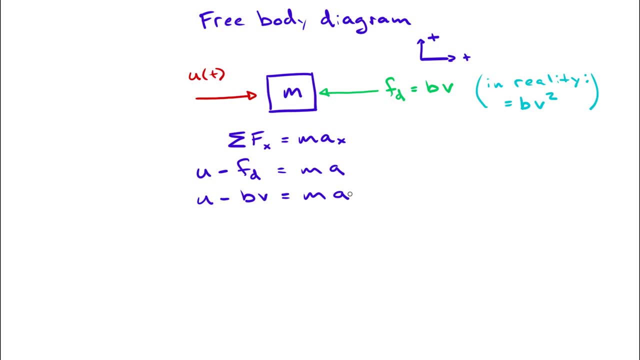 For example, we can think about this equation as an input-output relationship, where the input is u and the output is the velocity v. Thus our equation should be: in terms of these variables, Making the appropriate substitutions, we arrive at the following ordinary differential equation: 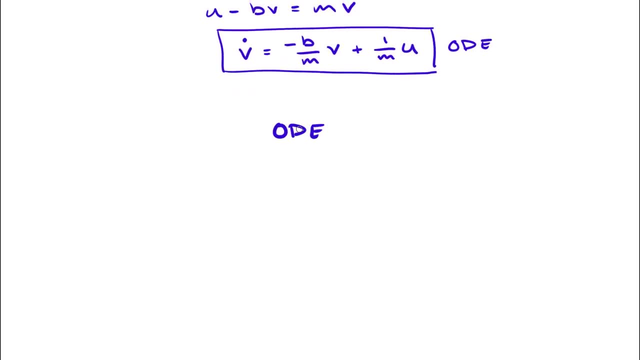 It's important to pause at this moment to understand what this equation represents. It's a mathematical representation of the dynamic system defined in the free body diagram. In other words, for any given input and output, we need to understand what this equation represents. 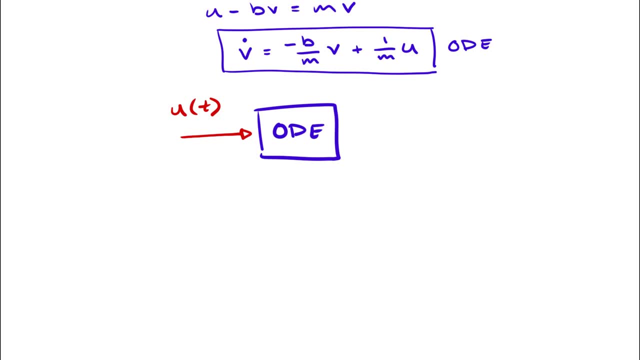 For any given input, u, we should be able to solve the differential equation and arrive at the actual output velocity profile. Let's use one example to verify our intuition at the very beginning of this video. If the input has the form u equals 1,, in other words, just a constant value, then the particular solution to the differential equation has the following form: 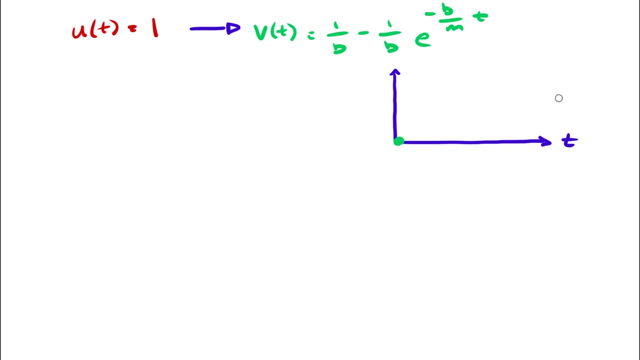 It's clear that when t is equal to 0,, the velocity is a constant value. It's clear that when t is equal to 0, the velocity is a constant value, But if it is equal to 0,, the velocity is also equal to 0.. 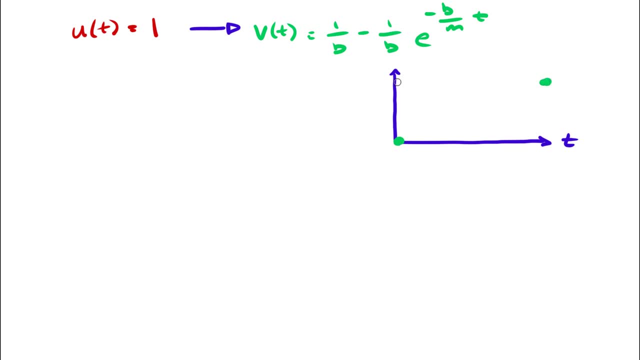 But if it is equal to 0, the velocity is also equal to 0.. Additionally, when t approaches infinity, the velocity approaches a terminal velocity of 1 over b. Additionally, when t approaches infinity, the velocity approaches a terminal velocity of 1 over b.